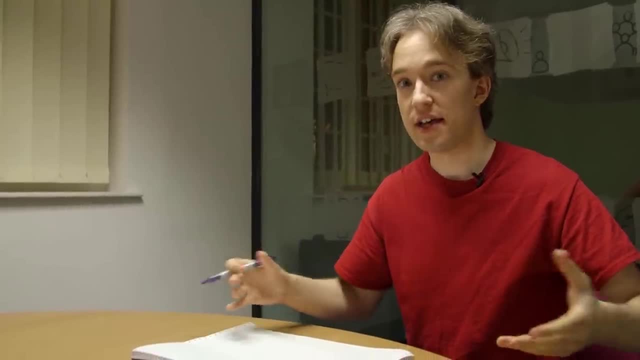 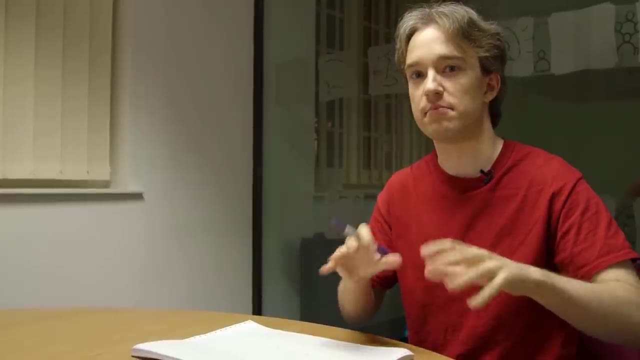 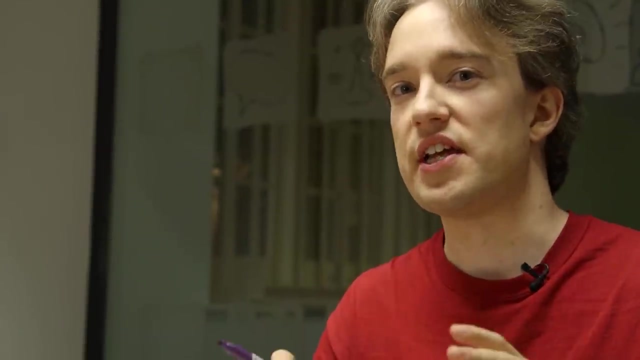 Cross-site request forgery- CSRF- is the third big web attack. I've talked about cross-site scripting in the past. I've talked about SQL injection. this is number three and it's the lesser-known one. Web browsers are fairly trusting things. 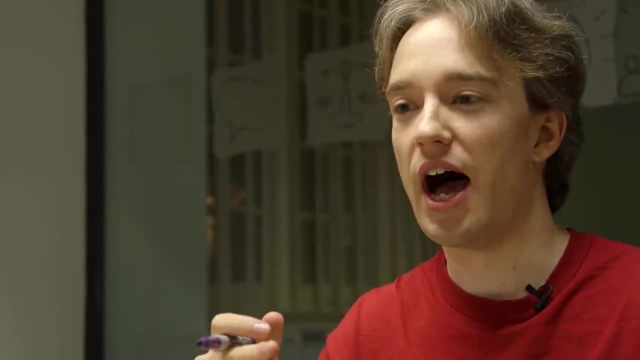 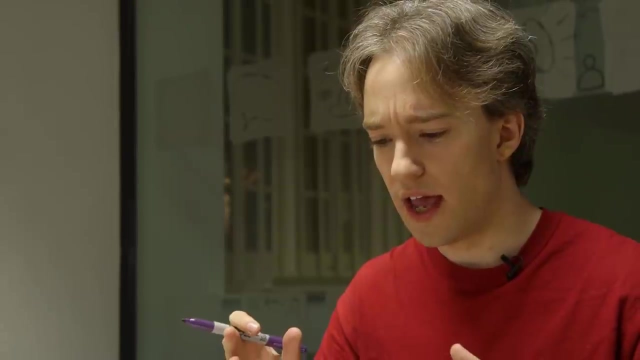 I've said this before: if you give them some code to run, they don't cast a value judgement on it. they can't tell if it's malicious, they will just run it. Now, this was kind of okay in the early days of the web. when there wasn't online banking and things like that, the worst you could do is put a comment somewhere. Nowadays, a bit more complicated, The web runs on data being sent back and forth, and that data can be encoded in a couple of ways. 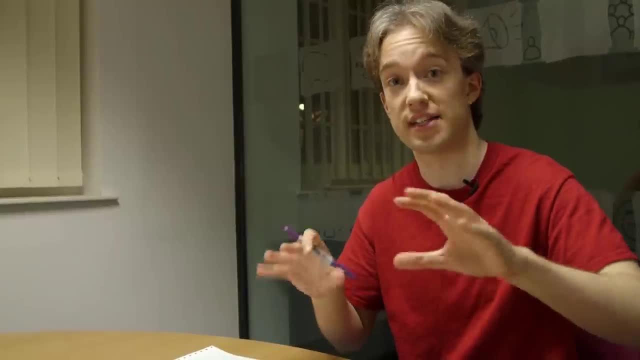 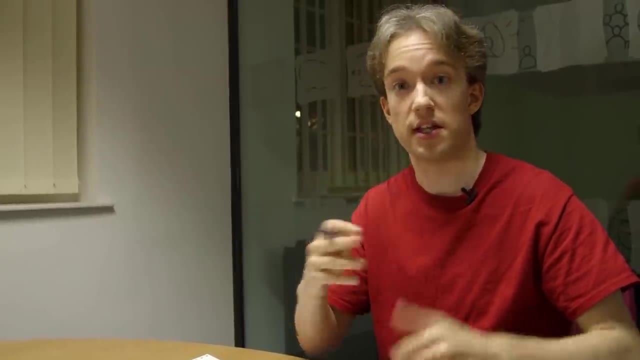 You can have what's called a get request and that's like, if you look up, if you're using this on desktop and you look up at the browser address bar, you'll see youtubecom slash watch. that's the name of the page. 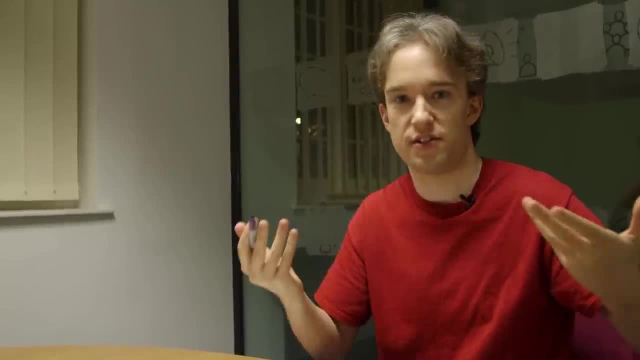 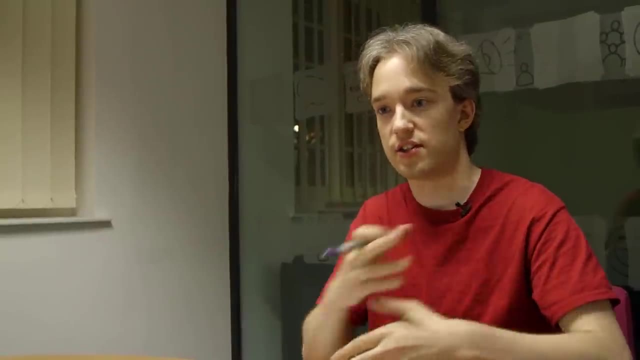 and then a question mark and then v equals a string of characters. That means that you go into the watch page and then the rest of that gets stripped off and sent to the logic at youtube which says: oh, we want this video to pull these details out of the database. 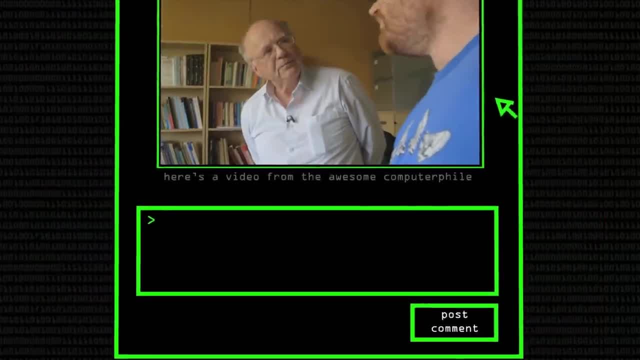 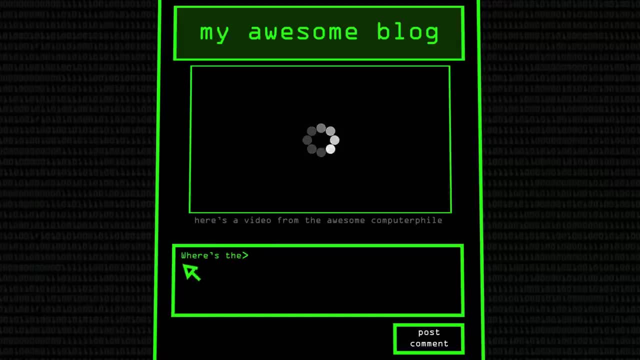 There's another way of doing that, called post, which is the kind of thing where you have a form with a button at the bottom of it And when you hit go, then all that data gets bundled up and sent along with the request, but not in the address bar. 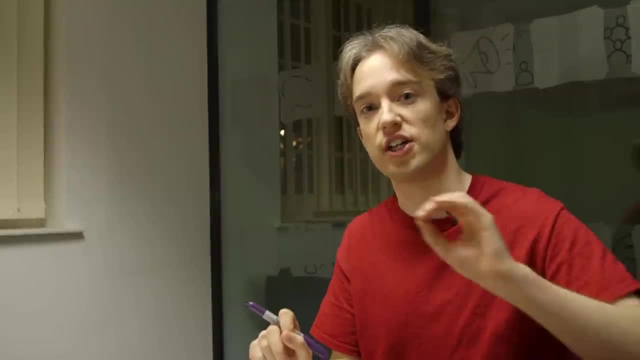 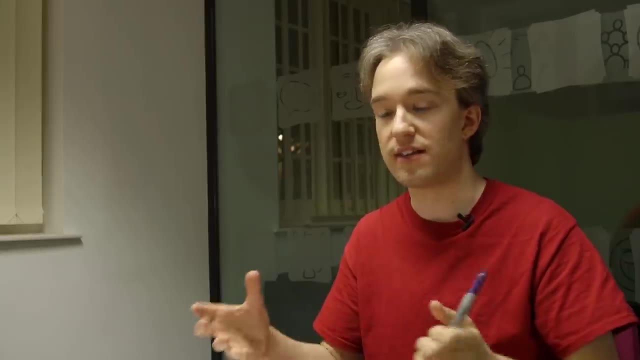 And traditionally, if you put it in the address bar, it's designed for fetching data. it's called a get. So that means that you can take this YouTube URL and copy and paste it to somewhere else And just bundling the data up, like when you click go on. a form is called a post. 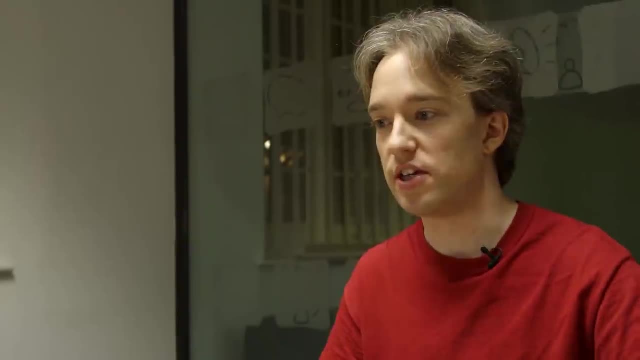 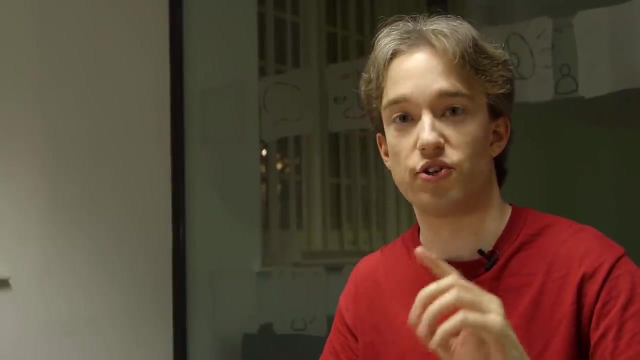 and that's meant for writing things, for things that happen once, so that when you hit refresh or go back to the same page it doesn't do the same thing twice. So if you enter a comment it doesn't put all your comments details in the URL bar. 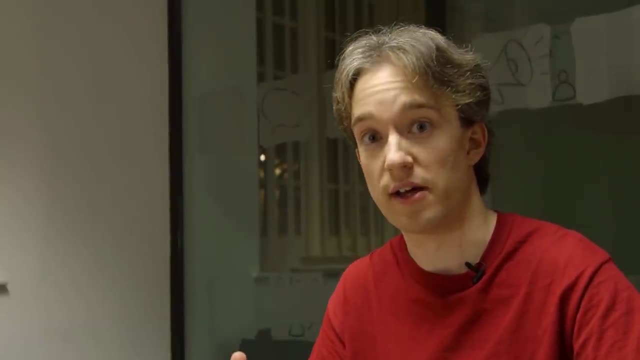 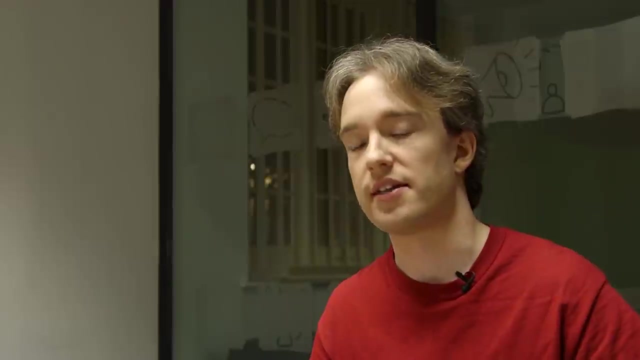 and you can't copy and paste that to a friend and they'll post the same comment. And that's reasonably good for the early days of the web. but since then it's got a bit more complicated. Let's say you have a form on your website for an online bank. 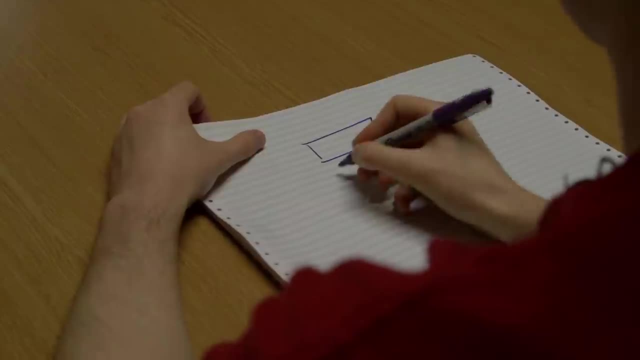 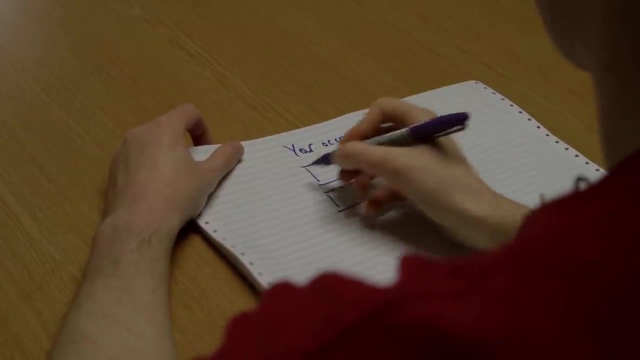 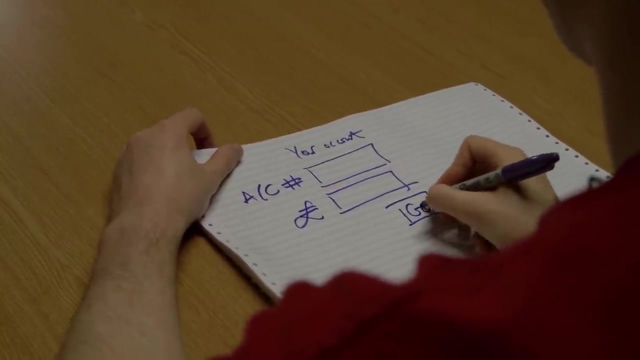 So let's design a really bad online bank form. Let's have send some money from your account to this account number and send this much, And then there's a go button And let's say that as long as you're logged in. 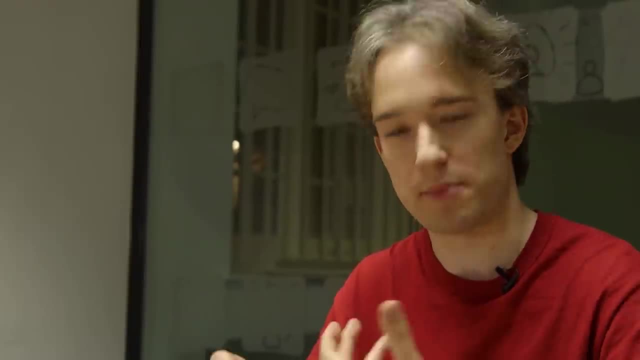 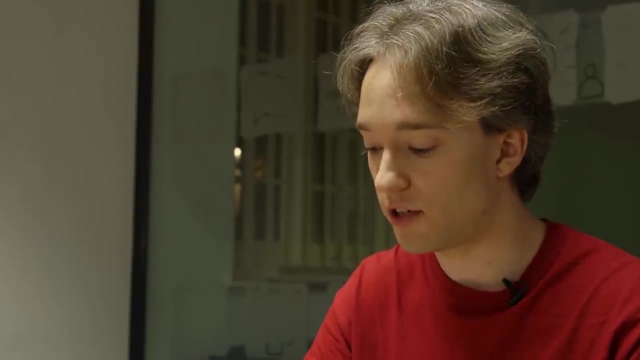 as long as you've been through all the authentication checks and used that little chip and pin device that gives you a password to type in, you've got access to that form. You type in the account number. you type in how much you're transmitting. 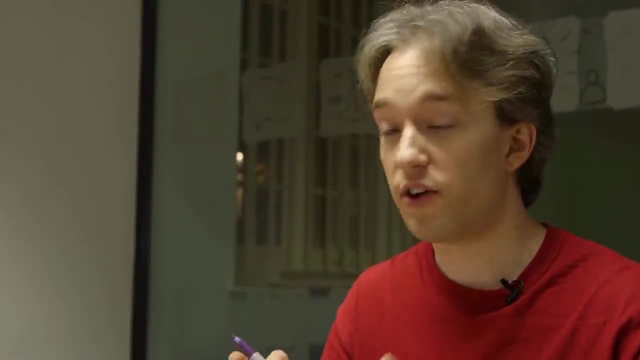 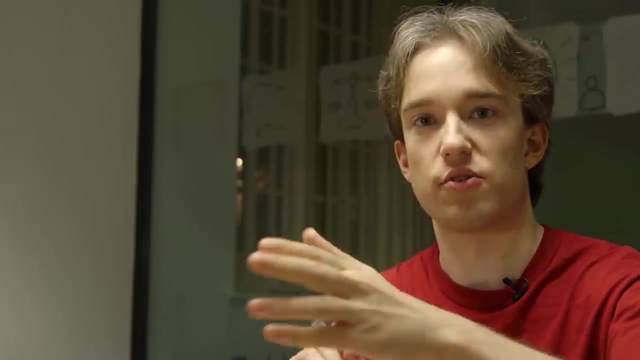 you select go. First of all, this won't use a get request. It won't appear up top, like YouTube does. It'll bundle it up as a post. it'll send the request and your bank will send back that it's done. 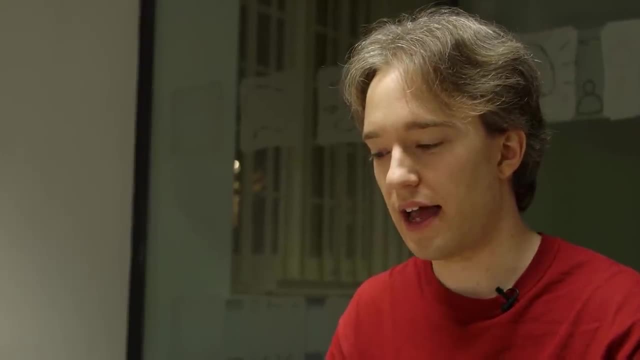 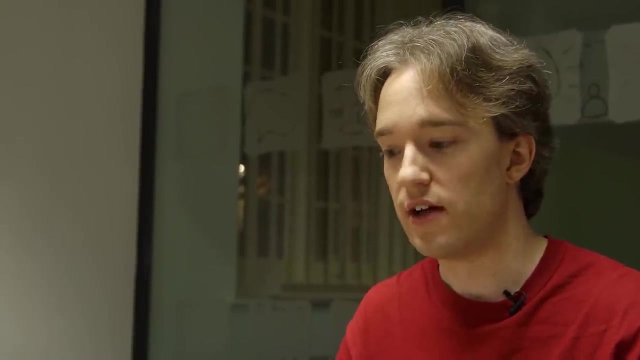 But the trouble is that form is, well, almost public. You know how it's designed. So let's imagine you set up a fake web page somewhere else that has that form on it And maybe, just maybe, you hide some of those details. 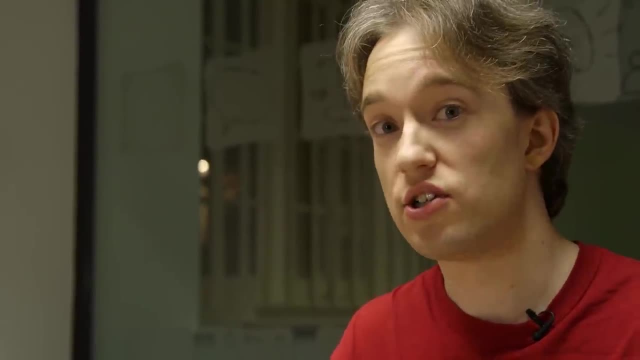 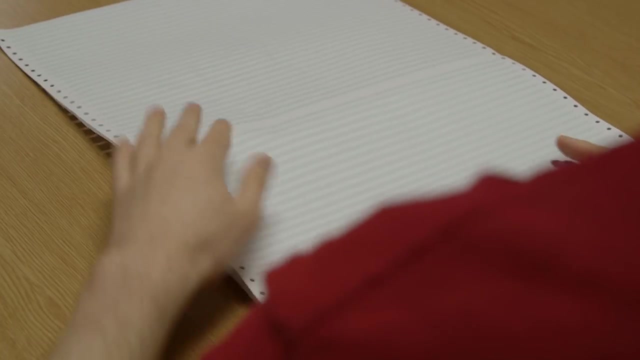 So they're already typed in, So it already has your account number in it and say a thousand pounds. And then when someone comes along and they want to put a comment on your website, so let's design a really malicious blog. 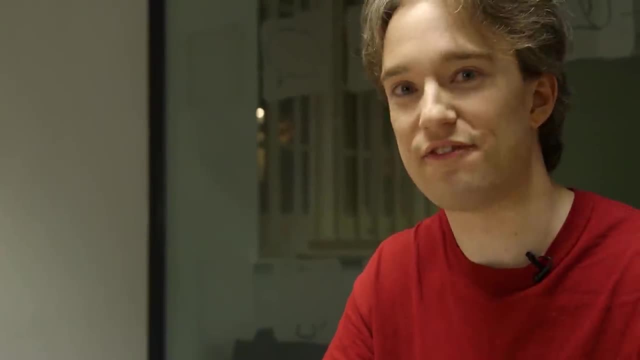 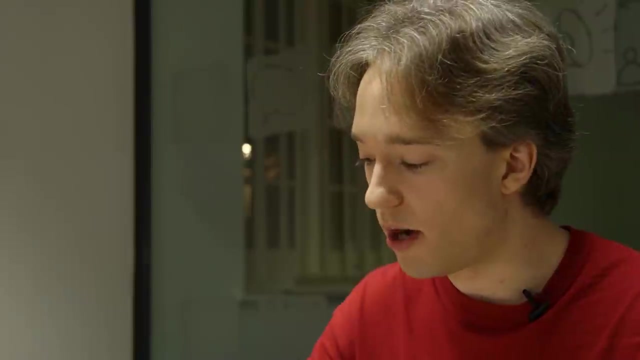 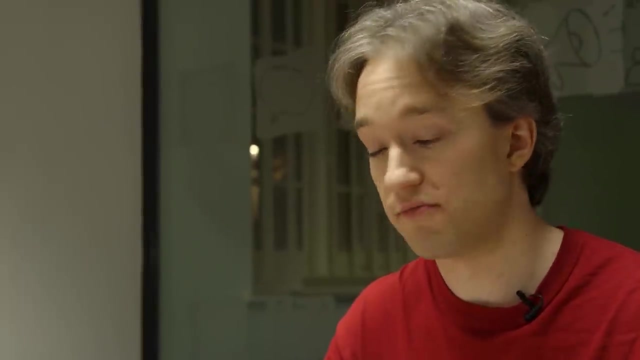 Let's call it My Awesome Blog and let's write some really inflammatory content that people will love to comment on. And here is a comments box. But off here, off-screen, where they can't see it or even completely invisible, is a box that says account number, pre-filled with your account number. 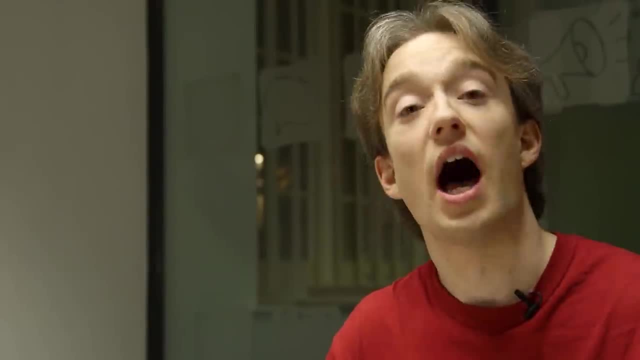 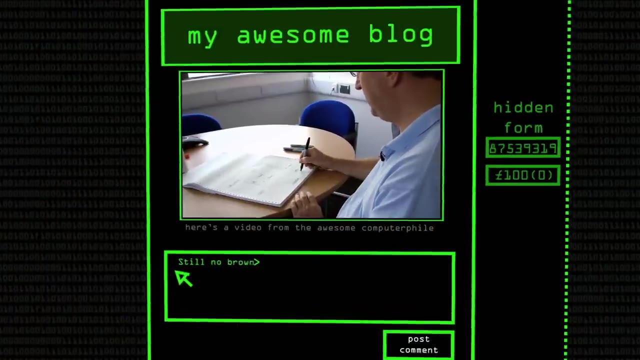 amount: a thousand pounds. I've written a hundred, A hundred pounds because apparently my hand has lower ambitions than my brain does And when you click that go button it's not going to My Awesome Blog, It goes to the really badly designed online bank. 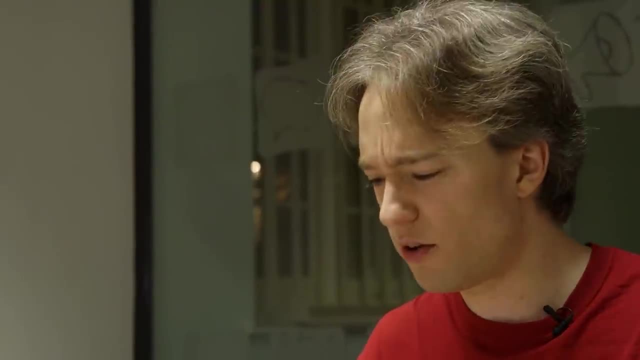 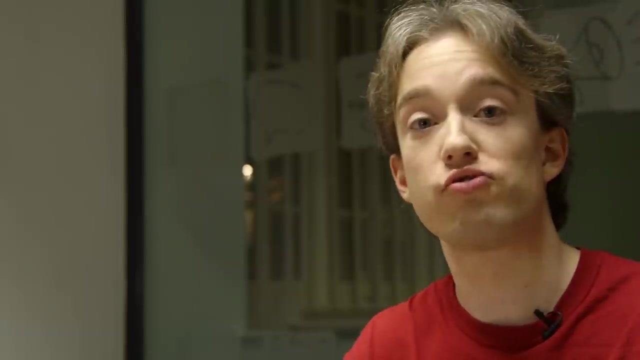 Which promptly says: oh, we've got a request here. Don't know what all this blog nonsense is about, but look, we've got an account number. We've got some money. Transfer it Because we've already been authorised, Because you're logged into your online bank in that other tab while you were bored. 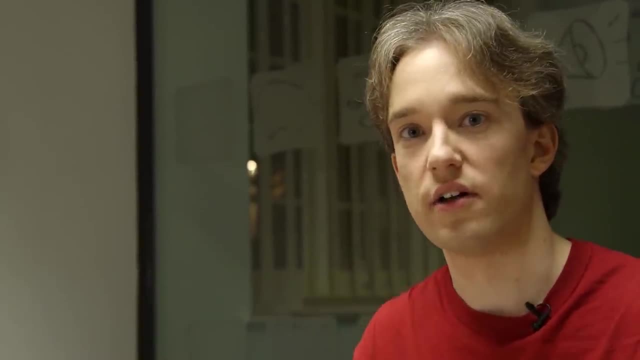 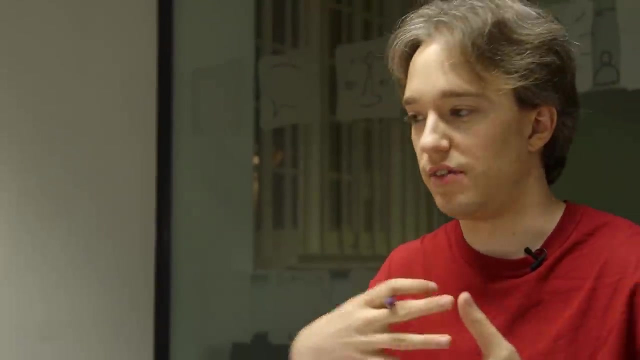 And well great, The money is gone. And it gets worse than that because, if you've noticed, when you type a comment on YouTube and you click post, it doesn't load the whole page back like it used to in the early days of the web. 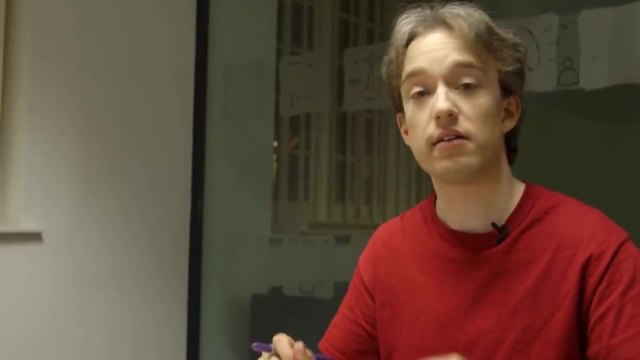 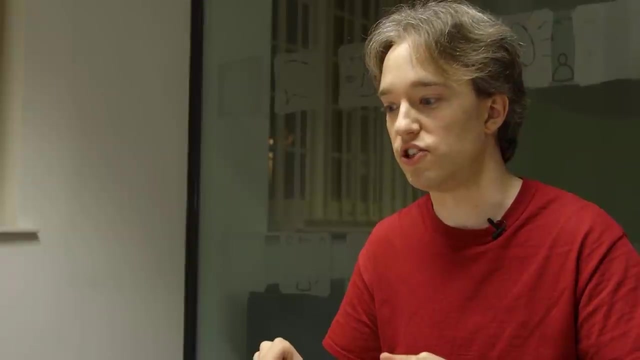 Now it does it all in the background, silently, and just sends a thing back saying, yeah, that's fine, no worries. Well, that would work with this too. You wouldn't even need to click the go button. It could just be that when I load up my site, 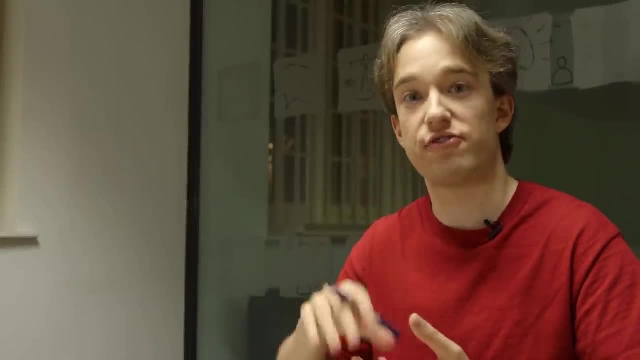 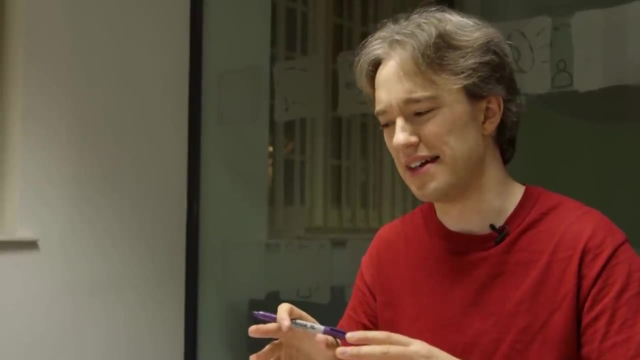 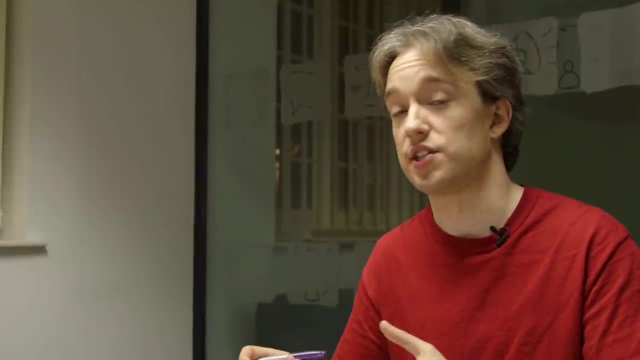 my malicious awesome blog. it just creates that form in the background and sends off that request. There's a few things in browsers designed to stop you doing that, but there are ways around them. Now, that's obviously quite a big problem. Online banks are generally not designed that way. 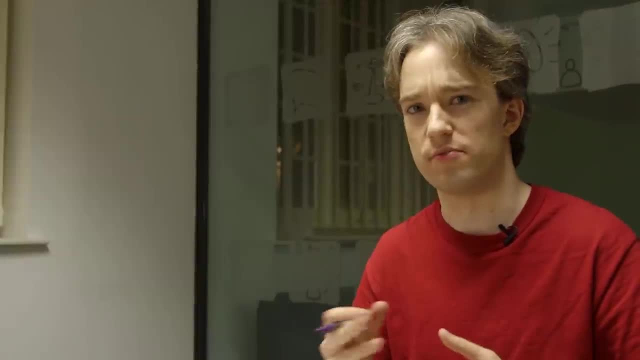 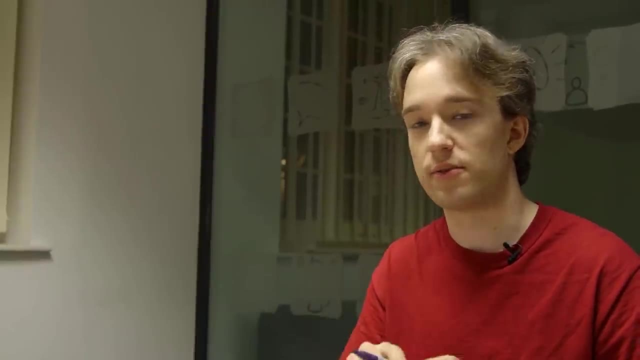 unless they're designed incompetently. But a lot of web forums, a lot of smaller sites have problems like that. If you've ever designed something with a delete your account button, then frequently it just goes to something like slash delete with maybe you know, confirm true on it. 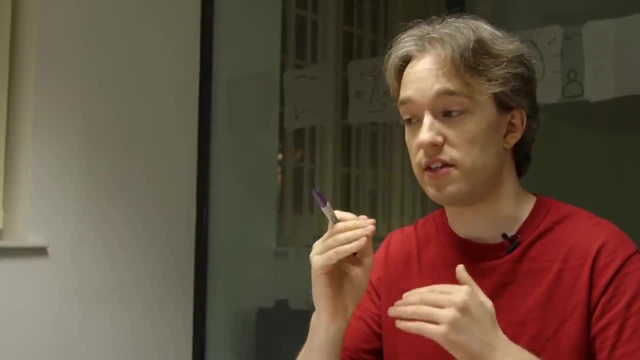 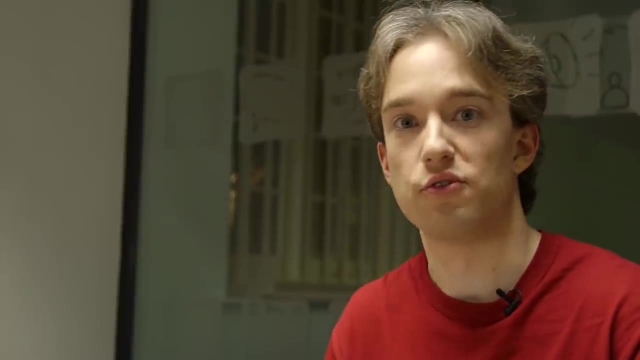 And you assume that the only time that form will be visible is when the user is logged in And has clicked. no, I really want to delete my account. I could copy that delete your account form and just put it in the background of my completely irrelevant web page somewhere else. 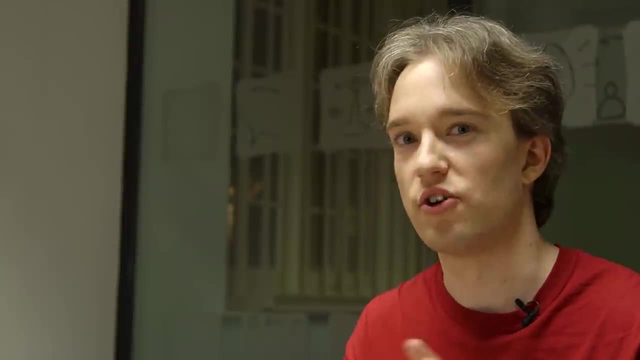 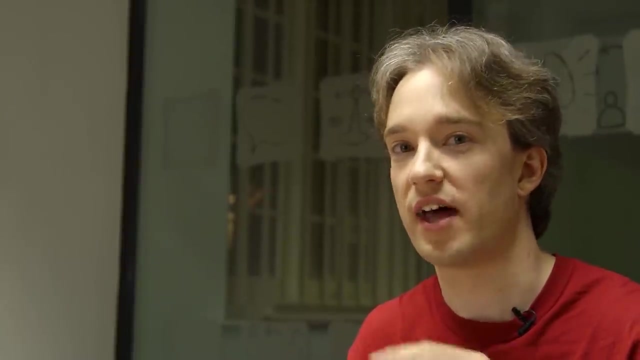 And you wouldn't even see that it had fired, because it's all happened in the background using modern web technologies And you wouldn't notice It would delete your account quietly in the background because that form that delete your account form or that transfer the money form. 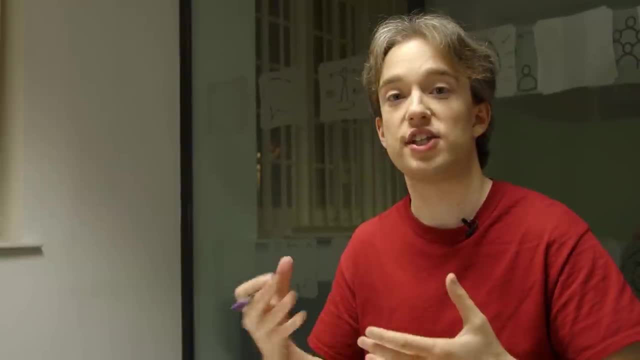 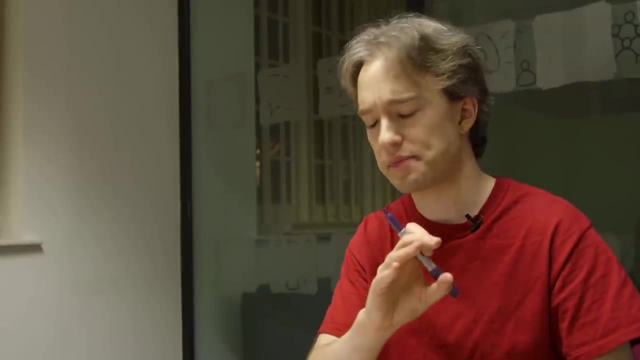 hasn't checked where the request is coming from. There was something in what's called HTTP, the hypertext transfer protocol- the very basics of the web- designed to stop this, And it's called the referrer header And it means that when you click a link or submit a form, 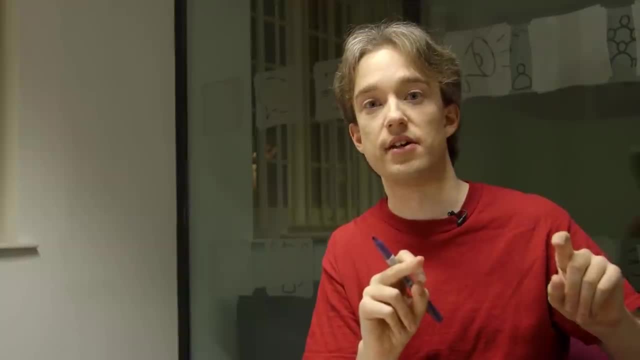 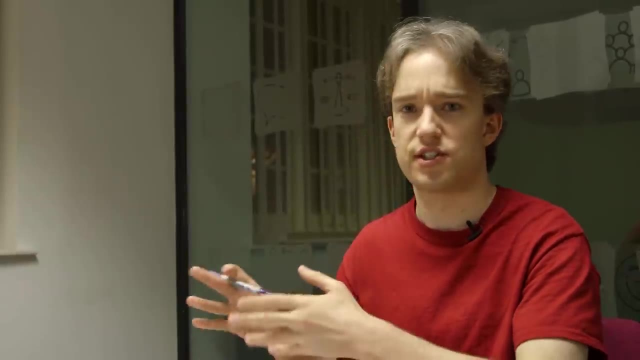 it includes a thing that says referrer this site, So you know if the form request is coming from the actual online bank or the actual delete your request form and not some malicious site elsewhere. The trouble is if you start checking for that. 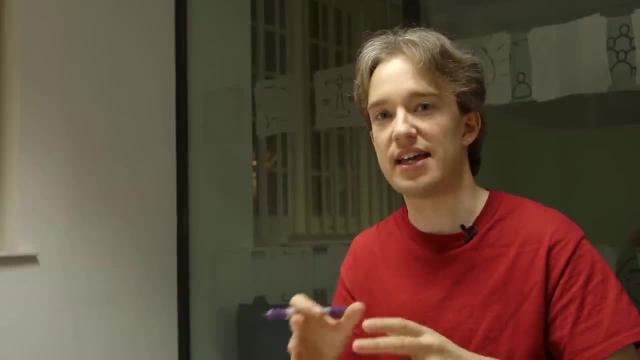 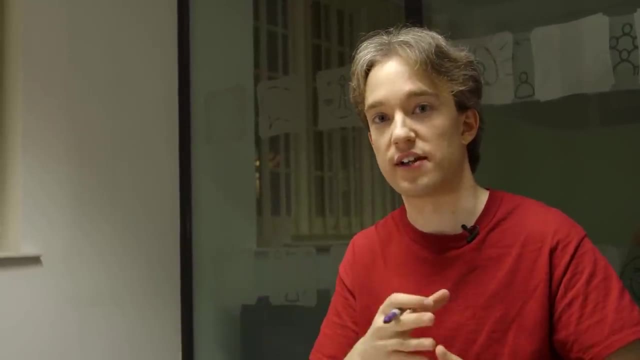 a lot of users start complaining because that referrer header isn't always sent like it should. Maybe you've got an advert blocker, or maybe you've got some kind of privacy tool that's blocking that as well. The way to get around that is a one-time key. 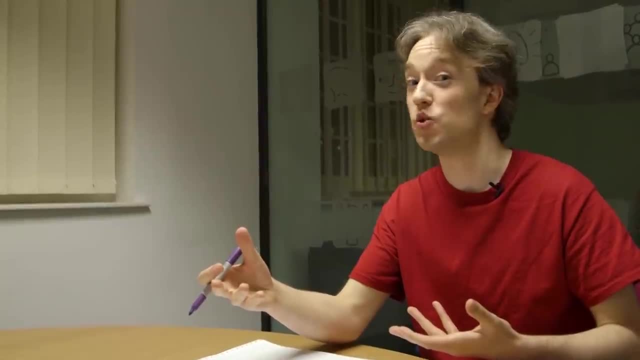 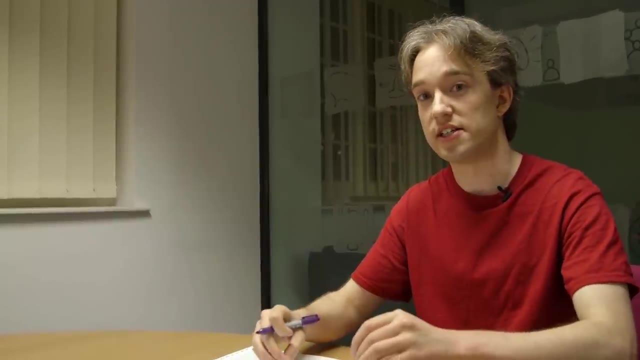 What the Americans call a nonce and which the British definitely do not call a nonce. The one-time key works by the form on your website, generating a unique code. It can be anything, just a random string of characters each time you create the form. 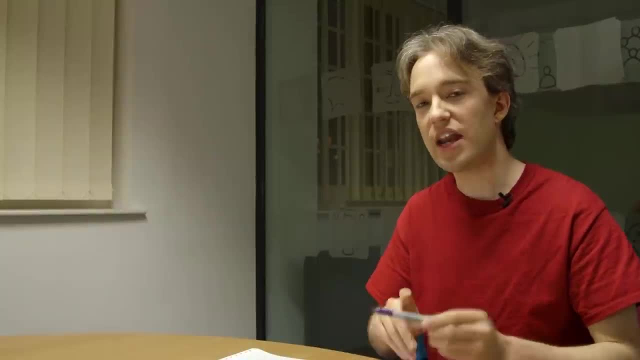 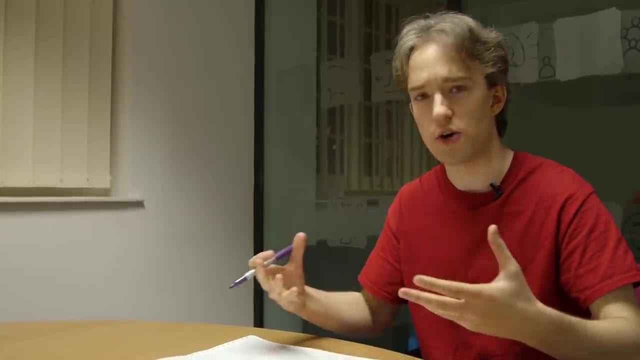 And then storing that character and saying: right, anything that comes back, anything that I see needs to have this token with it. And this code, this token you've generated, is in the form as well, Completely hidden, invisible to the user. 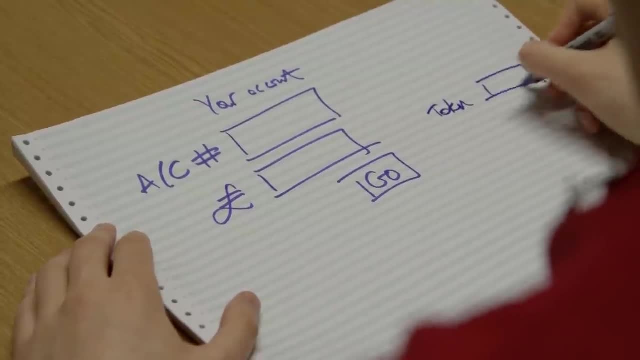 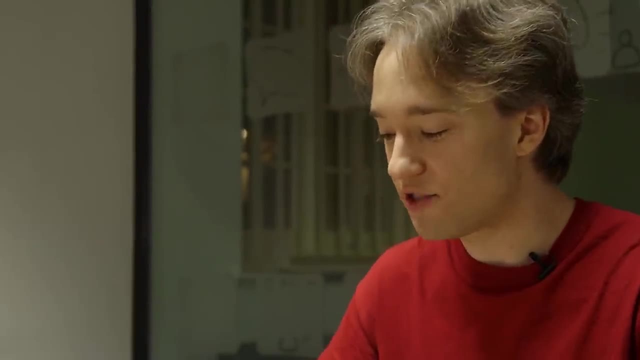 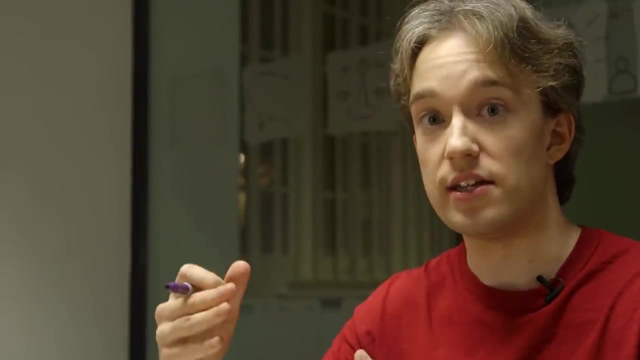 is something that says token, random string of characters. I think I just wrote a number plate. This random string is meaningless, but what it represents is that this form that I just made and I just sent out to the user is the one that's coming back. 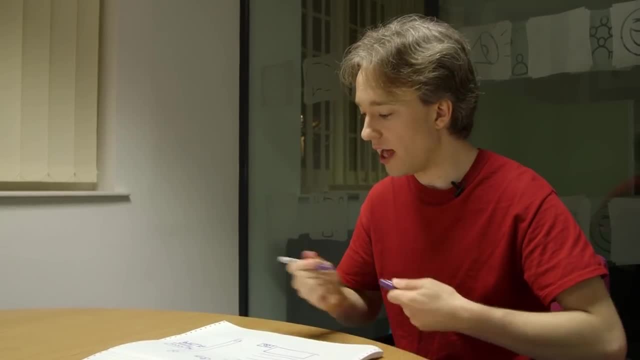 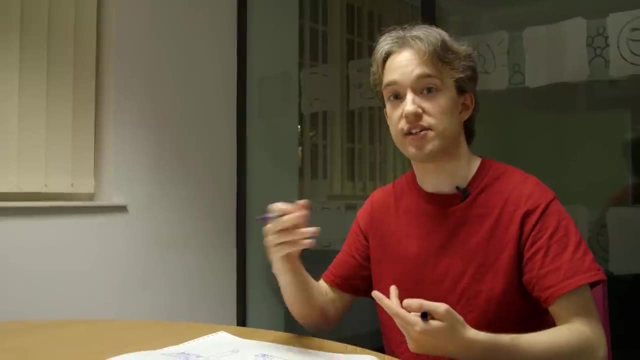 So meanwhile, over on my malicious awesome blog. I don't know what this token is. I can't possibly know what this token is because it changes per user and it changes every time the form is requested, or at least every few minutes. 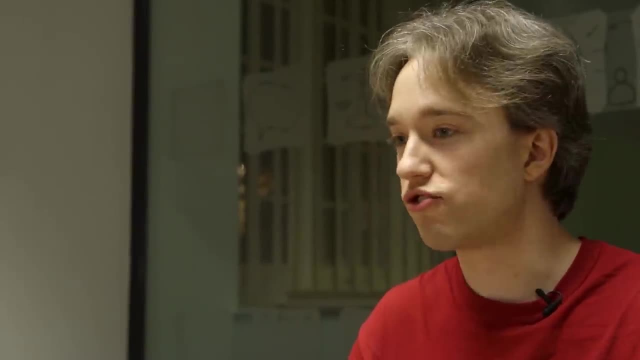 And if you copy that form, if you take that token and try and use it five minutes later, or ten minutes later, or on a form that's already been submitted, or for a different person, or for any one of these things? they'll look at that token and they'll go: that's wrong. I'm not having that. And suddenly cross-site request forgery doesn't work anymore And there are still theoretical attacks and lucky flukes that could get past this. 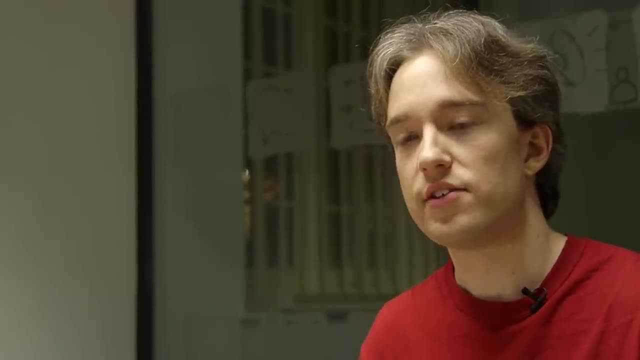 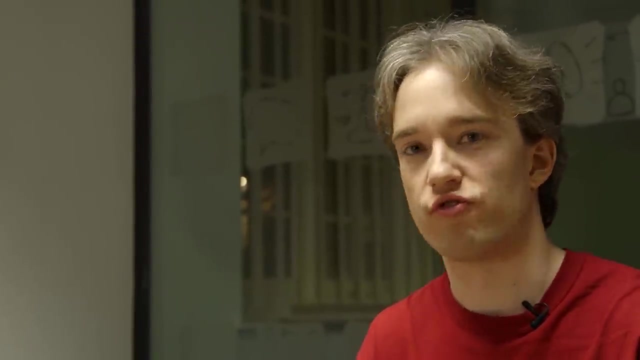 but in general, that solves it. So if you're designing web forms for anything which is permanent- anything like deleting an account, posting a comment authorising someone or even transferring money- if you're not using this, this is a pretty big security hole. 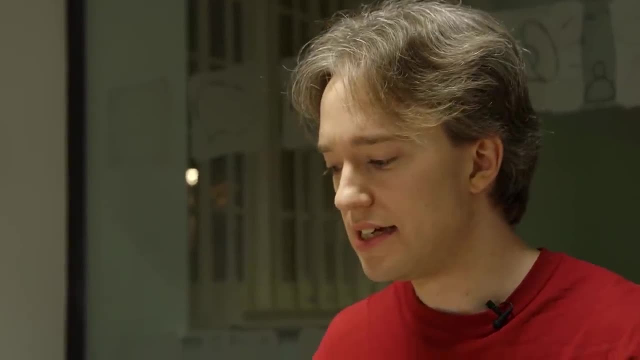 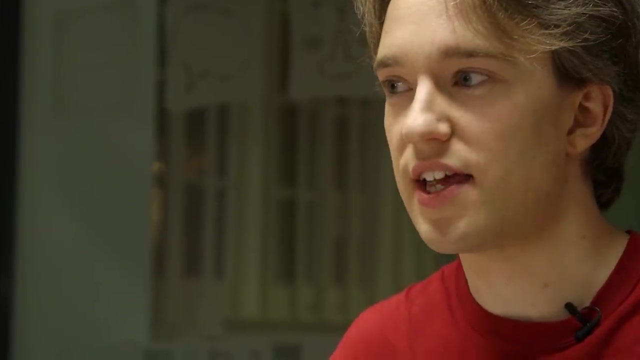 And if the sites you're using aren't using it, well, you never know what might happen when you go to some malicious blog somewhere out there. So that's cross-site request forgery and it's the third attack, And everyone knows about XSS. 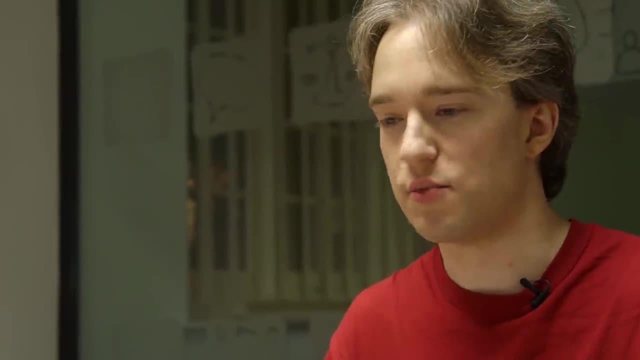 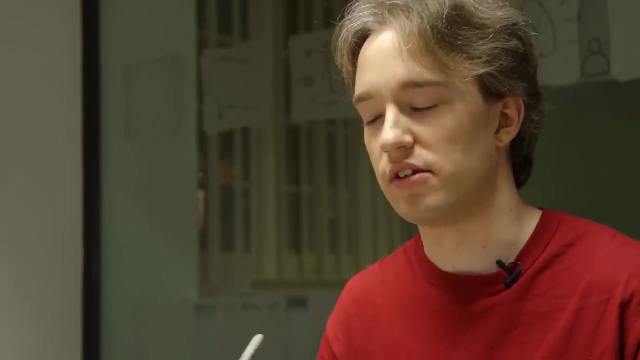 If you're a web developer, cross-site scripting, XSS is the one you know about. SQL injection, database attacks are the one you know about, But this, This one, went under the radar for a long time, and there's still a lot of developers.